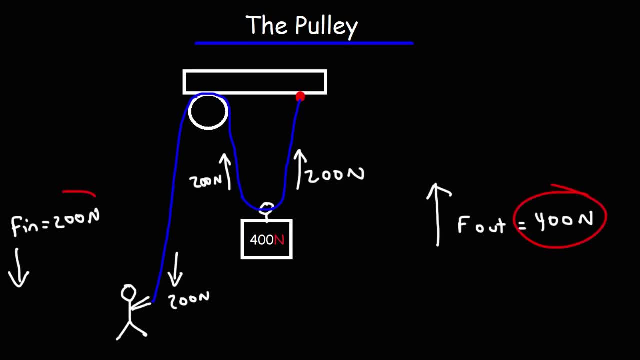 The ratio of the output force divided by the input force is two, And that is the mechanical advantage of this particular pulley system. It's equal to the output force divided by the input force, And that's the purpose of this device. It allows us to multiply the force that we input to this machine, making the work a lot easier to do. 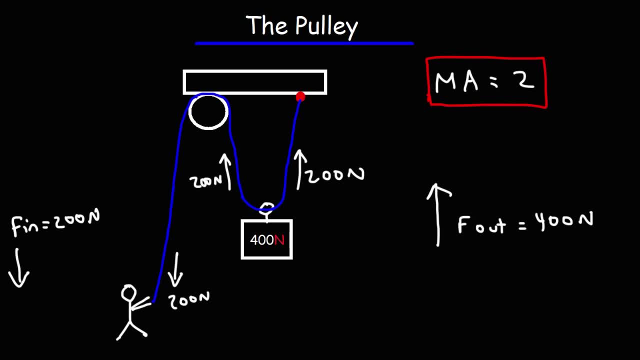 Now there is a cost to pay. This multiplication of force does not come free. In order to lift up the crate by a distance of one meter, the person has to pull down the rope by a longer distance of two meters. Why can we say that? 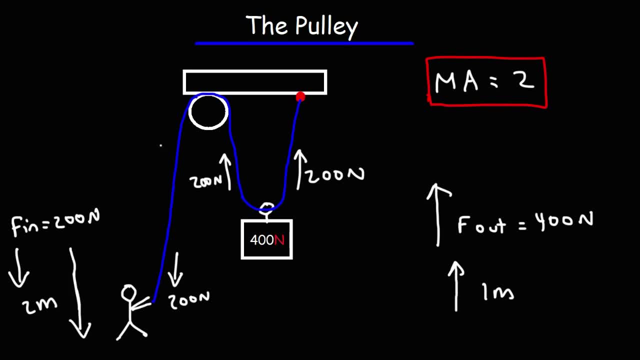 Well, as he pulls down this rope by a distance of two meters, this rope is going to go up by one meter, Because this rope is going to go up by one meter. So one meter plus one meter equals a change of two meters on the other side. 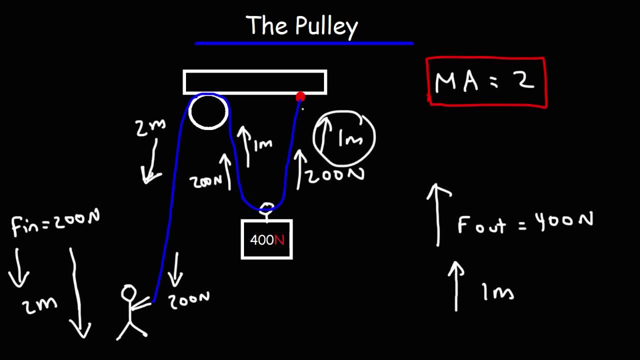 So if this goes up by one meter, the distance here decreases by one meter And this part is going to decrease by one meter. So this has to increase by two meters because the rope is not going to gain or lose length by any chance. 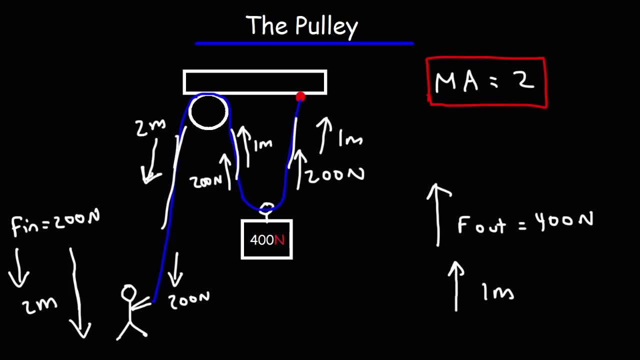 If these two ropes go up by a total of two meters, then this rope has to go down by a total of two meters. They have to add up and be equal to each other. Now, if these two ropes go up by one meter, 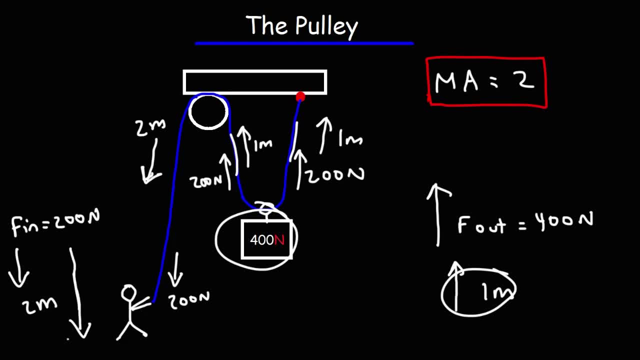 that means that the crate only moves up by one meter And in that sense there's a change in distance. So when a person pulls down a rope two meters, the crate goes up by one meter. Now let's calculate the work. 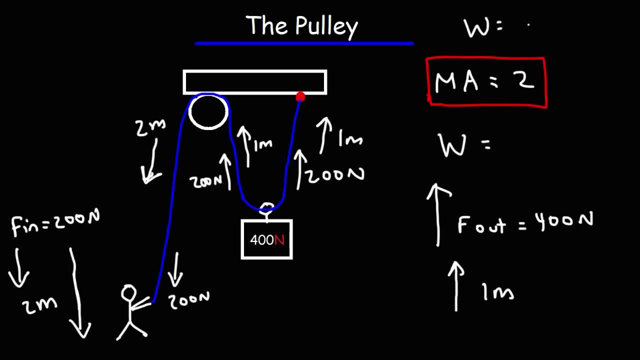 Work is equal to the force times the displacement. So we have a force of 400 newtons and the crate is being displaced one meter higher. So 400 times one we're applying 400 joules of work on this crate. 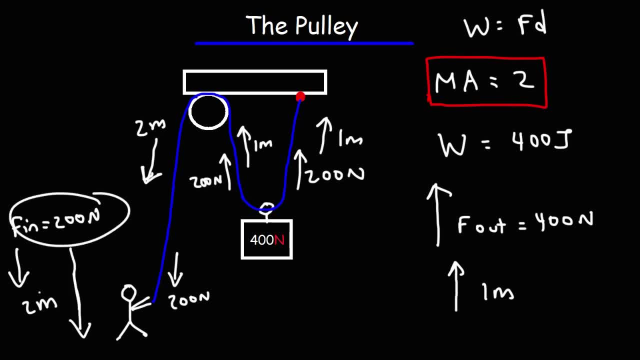 Now the person is applying a force of 200 newtons for a distance of two meters, So 200 times two the work that he's applying is 400 joules, So the pulley doesn't change the amount of work that needs to be done. 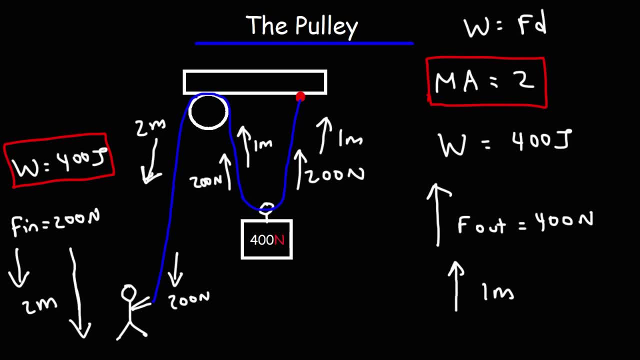 However, it simply changes the force that you have to apply by changing the distance. So, because the person pulls the rope for a longer distance, he can apply a much less, a lower force in order to lift the crate over a short distance. 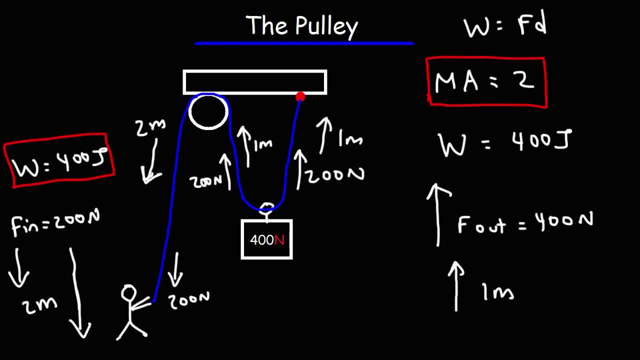 And so that's how these simple machines can multiply the force that we need to get the work done. It's by changing the distance over which that force is applied. So if we want to create a large force acting over a shorter distance, 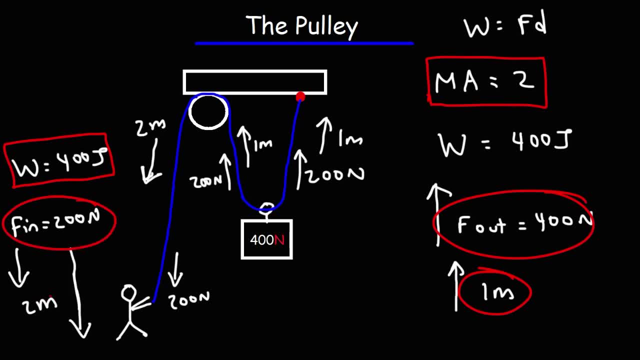 we need to apply a small force over a longer distance, And that's the principle behind these machines, how they work, But the energy that's needed to get the job done is the same. Energy is neither created or lost in this process. 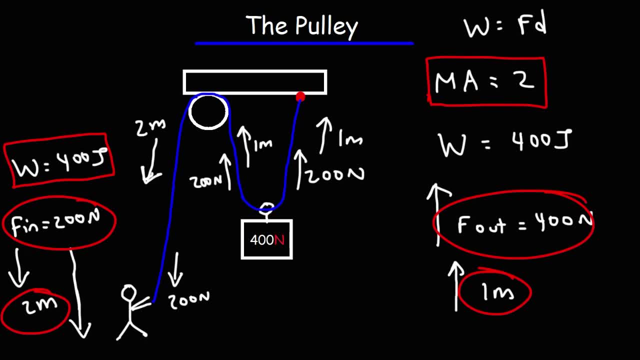 So the law of conservation of energy is consistent with this device. Energy is not created or destroyed here. Now there's something else that you want to take into consideration, And that is that the mechanical advantage of the pulley is equal to the number of ropes. 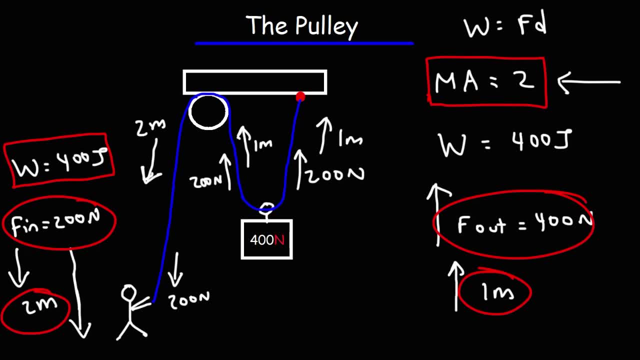 that is being used to lift up the crate. Notice that we have two ropes being used to lift up the crate, So the mechanical advantage is two. Now let's look at another example, but one that contains more ropes being used to lift up the crate. 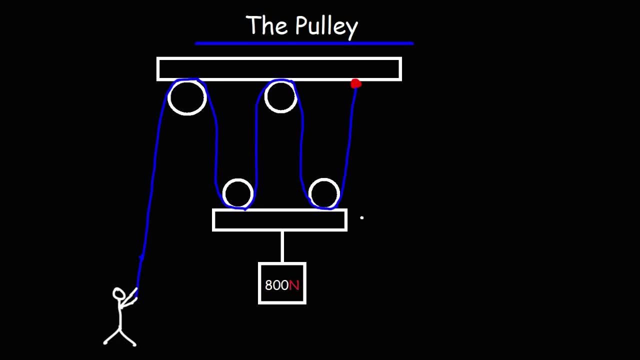 Now, looking at this pulley, what would you say? the mechanical advantage is: Notice the number of ropes that we're using to lift up the 800 newton crate. We have a total of four ropes being used to lift it up. 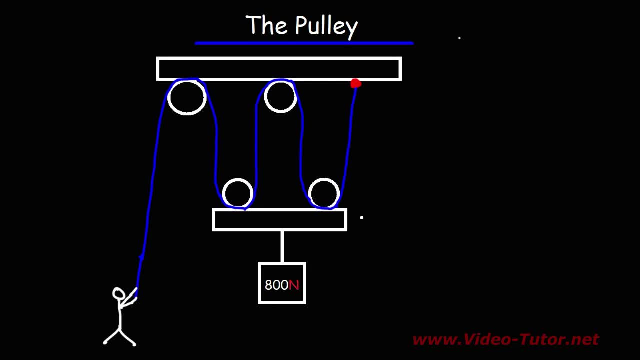 Therefore, the mechanical advantage is simply going to equal four. So just by knowing that, we know that the person is going to apply an input force that is four times less than the force we see here. So 800 divided by four. 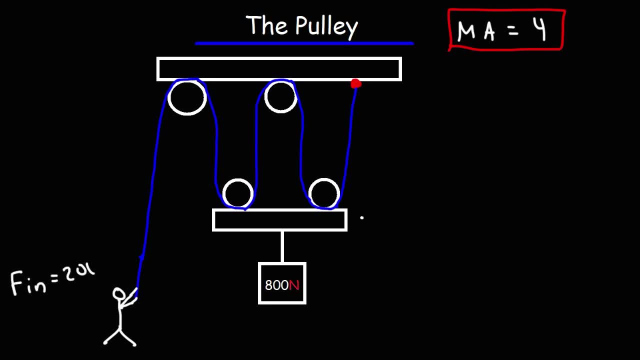 gives us an input force of 200 newtons. Now let's think about why We need to lift up a crate. that's 800 newtons, And all of the forces here in this rope are going to be the same. 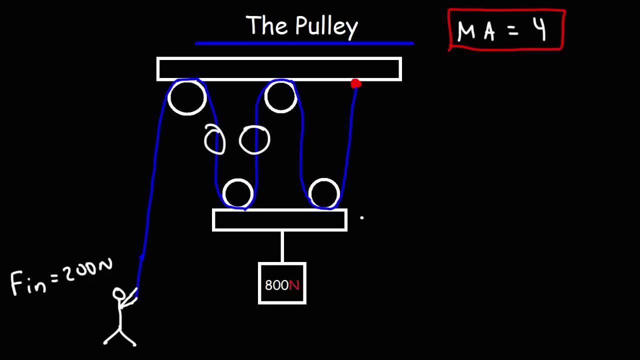 And they have to add up to 800.. So it's 800 divided by four, which is 200.. So this is going to be 200.. this is going to be 200.. 800.. and this is going to be 200. 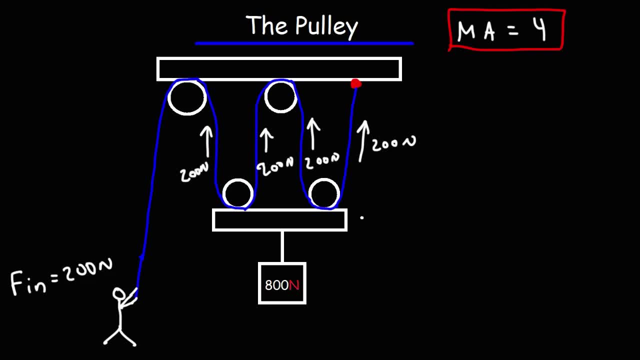 And that's 200 as well. So if you add up 200 newtons four times, you get a total force of 800 newtons. So thus the mechanical advantage is equal to the number of ropes being used to lift up the crate. 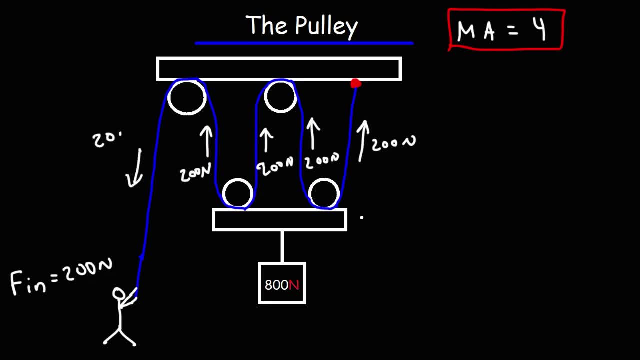 And, as we can see, the tension in the rope is the same throughout the entire rope. Now let's talk about the distance here. In order to lift up this crate- a distance of one meter- how far should the person? 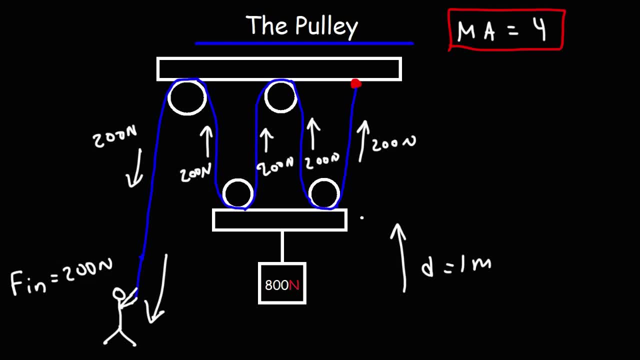 pull down the rope. Well, in order for the crate to go up a distance of one meter, each rope has to go up by one meter In an ideal situation. So we have four ropes going up by one meter. That means that 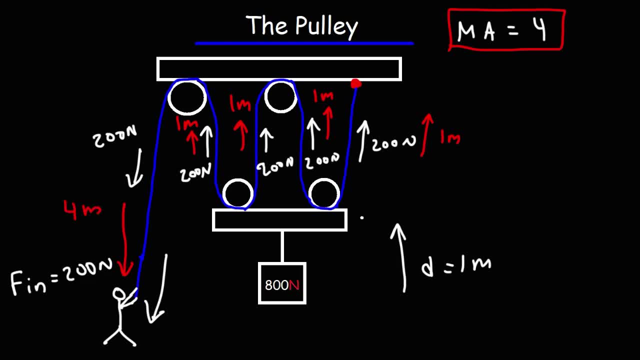 this rope has to go down by a total distance of four meters, And thus the work that is applied is equal to lifting up an 800 newton crate by a distance of one meter. So that's going to be 800 joules. 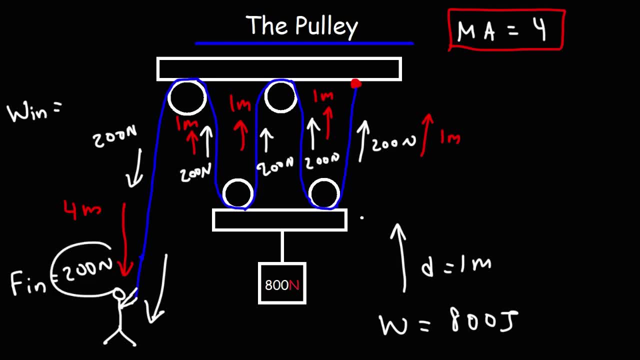 And on the input side we're applying a force of 200 newtons over a distance of four meters. 200 times four is eight. So we can see that the work that we apply at the input is equal to the work. 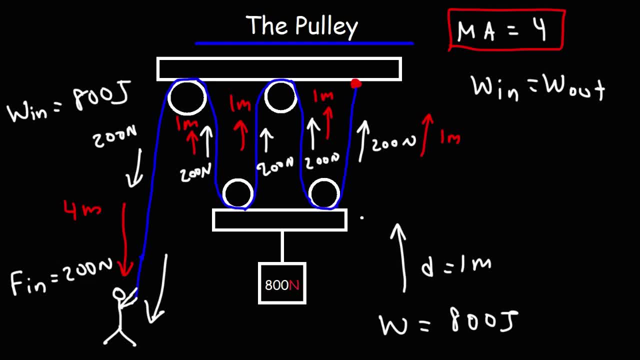 given a situation of 100% efficiency If no energy is lost due to friction or dissipated in the form of heat. Now, with this type of device, you can have any number of ropes that you want, If you were to use. 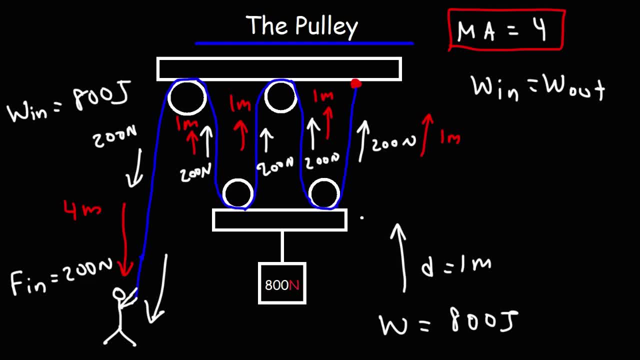 ten ropes, your mechanical advantage would be ten, Which means your force will be multiplied by a factor of ten. However, you will have to pull down the rope a distance that's too much. So by pulling the rope ten meters down,